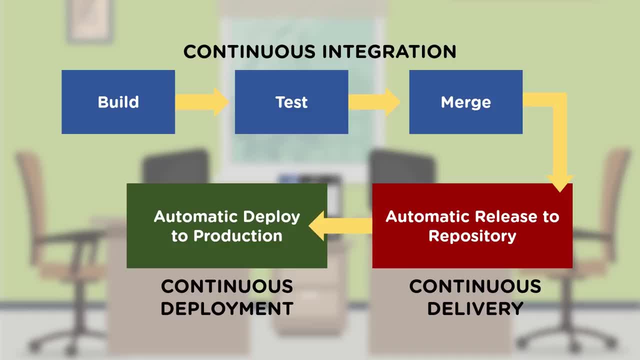 we need to proceed further or we need to halt there itself. So, after the continuous integration, the next process which comes into the picture is the automatic release to the rebooster tree over here, right. So it's just a kind of a mechanism where we will be releasing the source code to the artifacts. 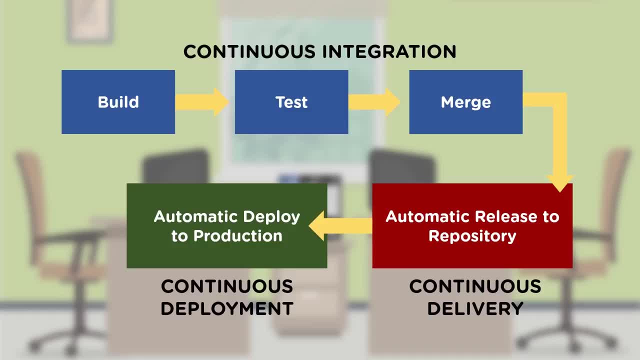 We are uploading the artifacts to the particular component, So that kind of automation is available. but that is also happening when we are saying that, yes, the test cases, execution Is successful and we have to proceed further, and at the end it's nothing but the automated. 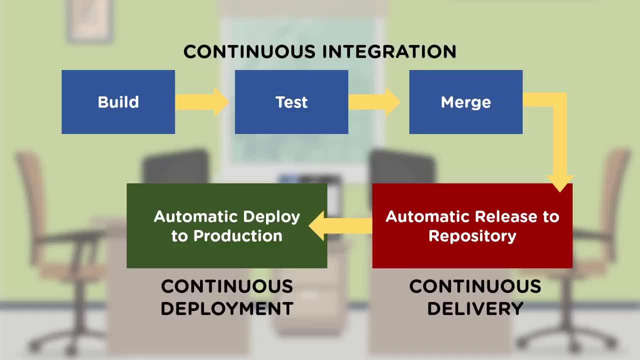 deployment to the production environment, which we call it as an kind of continuous deployment over here. So these are the overall process which we are looking forward so that we will be able to have an end to end automations going on over here with the help of CI CD automations. 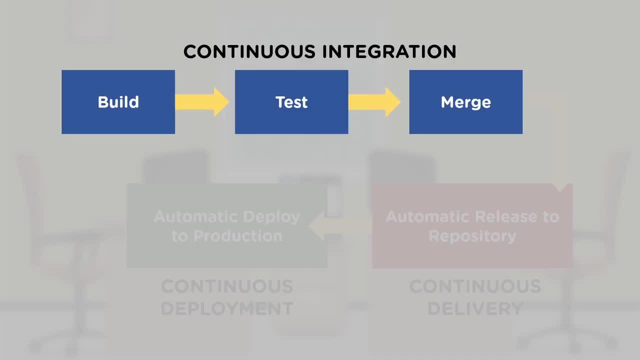 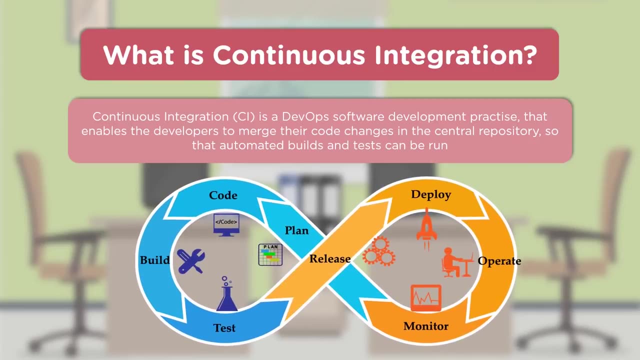 Now continuous integrations: again the build, test, merge. these are the different options which we do. So continuous integration is a kind of a process, a kind of a development process which is being used by most of the development teams nowadays. that eventually enables the developers to merge their source code. 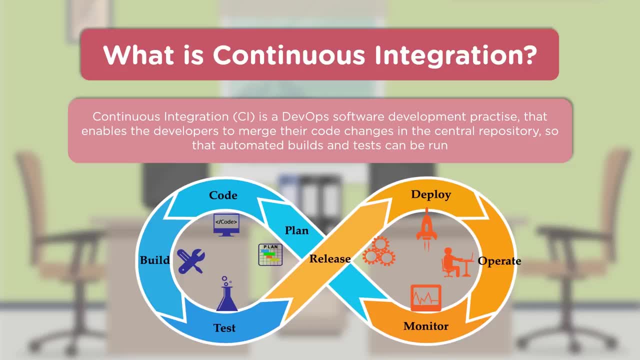 Whatever the changes, or whatever the modifications they are doing, they can- particular, you know like- merge their source code from their local systems to the central repository So that after that, with the help of CI tools, we can actually have the build automations and the test cases automation there. 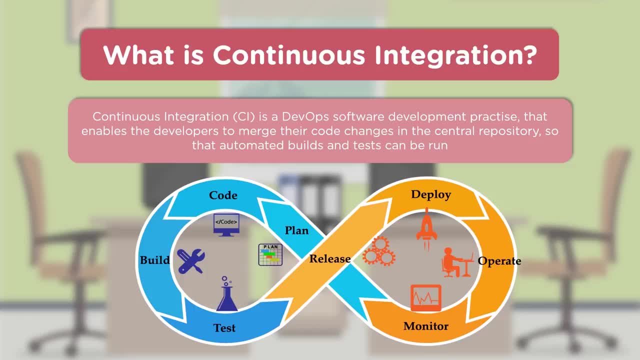 So this is the reason why we prefer the continuous integration process: because it depends on the basis of our modifications that how the whole build and test cases automations can really happen here Now. continuous integration is considered as a very important process because of the various reasons. 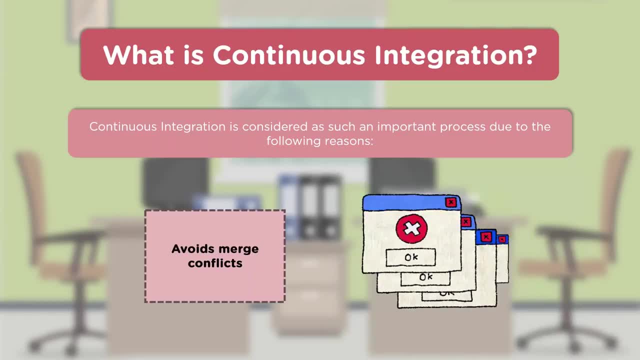 Let's talk about those reasons one by one. The very first one is that it avoids the merge conflicts, because if we frequently sync back our source code from our systems to the shared repository and the same thing can be done by other developers also, So eventually it definitely helps the different developers to collaborate their source code. 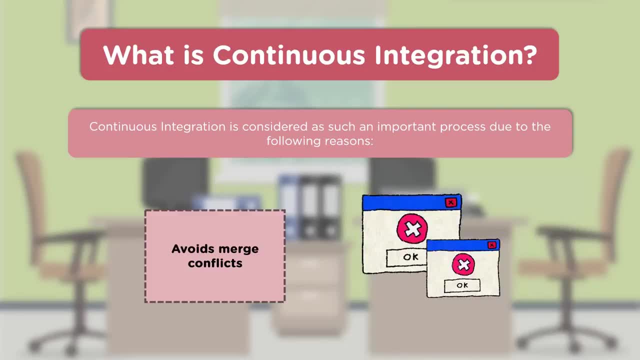 into a single shared repository and that can really help you to avoid the merge conflict situations, because you are always going to work on the latest source code, So the scope of merge conflicts is not going to be there. It also helps us to decrease the need of the code review because we are just doing the 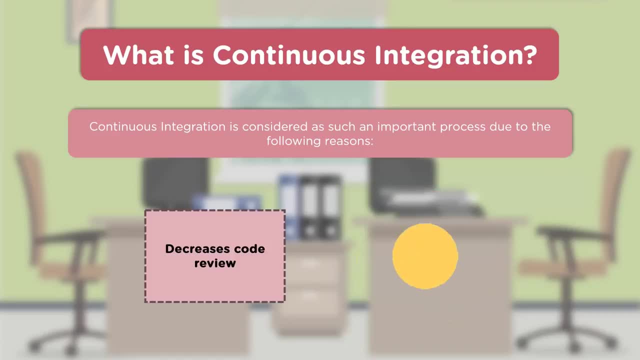 collaboration frequently, So we don't require any person to be sitting there and you know how to perform a kind of a heavy duty code review, because that is something which we can easily manage and we can work with that. So code review is something which we can easily decrease with the help of this continuous 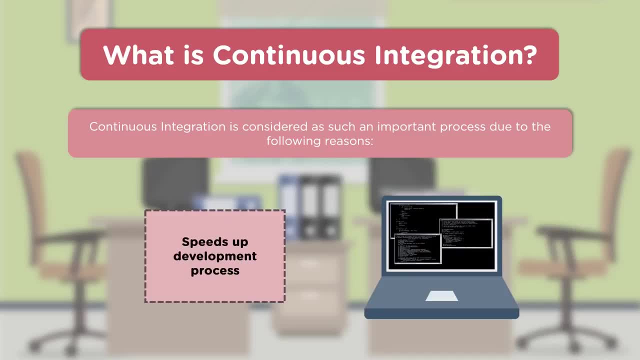 integration process. It also speeds up the development process. Yes, definitely, because the developers can easily collaborate with each other. So from collaboration perspective also, it's beneficial for us to do and that can really help us to see that, how easily we can integrate Our source code and that differs, or that basically helps us to go for the overall mechanism and 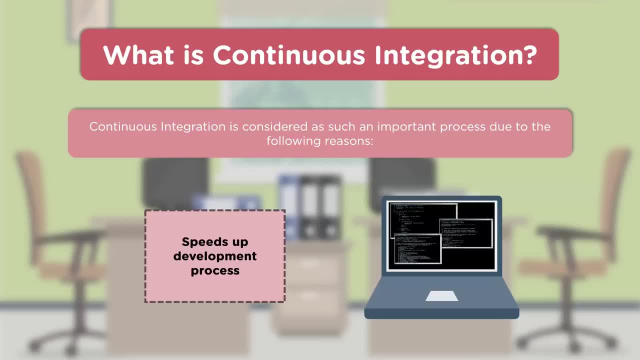 you know going for an perfect automation process over here, So it also increases the overall development process which needs to be implemented during the CI process. Next, it also reduce the product backlog, because we are doing our changes frequently into the repositories, So any kind of product backlog which is there, which is pending from long, that is also can. 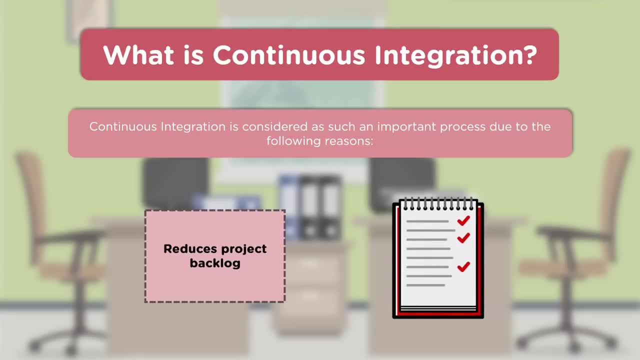 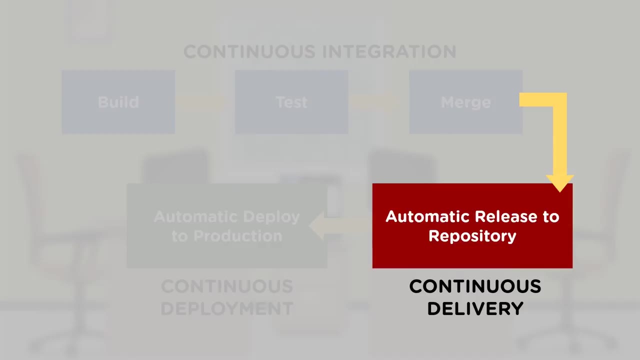 be managed easily Because it's keep on, you know, reduced there. So we keep, we keep on implementing our changes, we keep on implementing merging us particular changes to the shared repository So that reduces the amount of backlog which is available. Now next thing is the continuous delivery, which is an automatic release to the repositories. 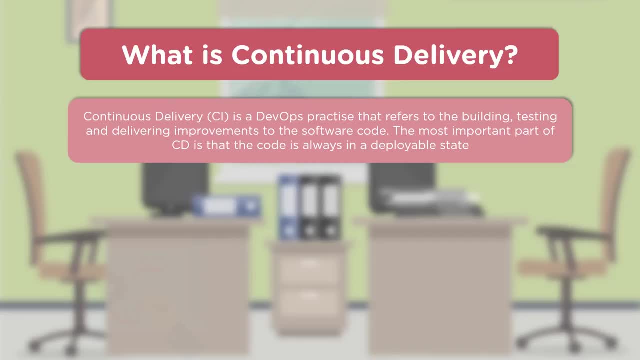 here. So what exactly is in continuous delivery all about? So continuous delivery is a kind of a practice that refers to the particular building, testing, delivering improvements to the software For code. So the important part of a continuous delivery is that the code is always in the deployable. 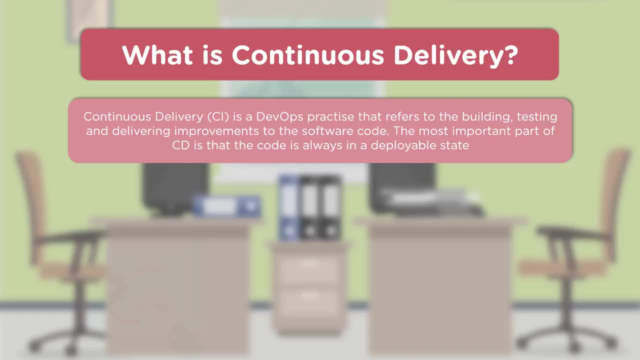 state. So we are saying that we are done with the delivery, we are ready with the delivery and whichever environment, whichever particular server you want us to deploy, we are ready to do that. So that is where we call it as in continuous delivery. So we have our artifacts ready and whenever is desired, whenever we feel that we want to. 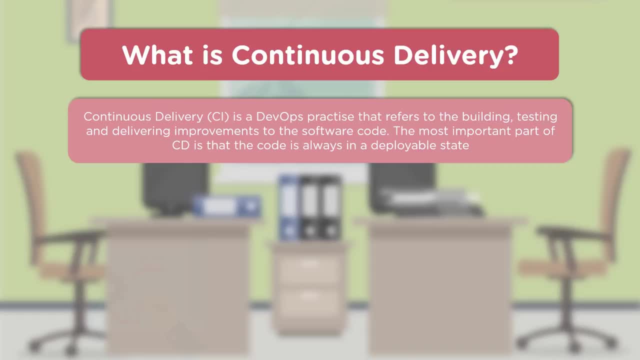 do the deployments. we want to proceed further. we will be able to do that with the help of this process. So it's in kind of an end to end process. You do the builds, you do the test cases executions. once the test case execution is done, once. 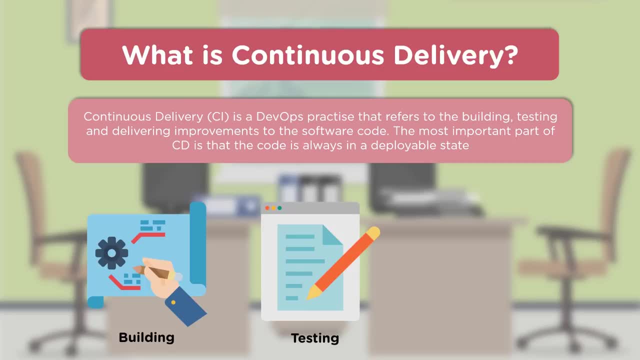 the testing is done, then you create an artifacts. you create a particular var files, jar files, er files, whatever the artifacts we have. we prepare that artifacts and then we deliver it to a specific environment. We say that, yes, let's go with the delivery, let's make it into a particular state where 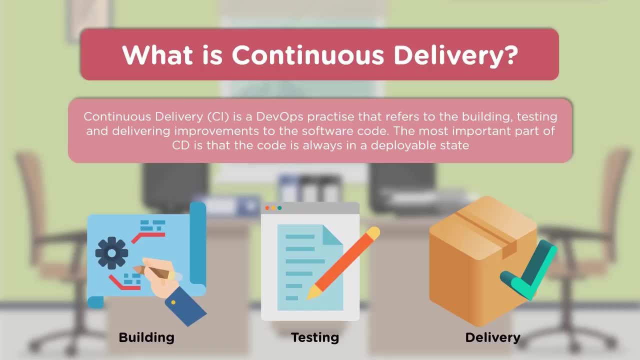 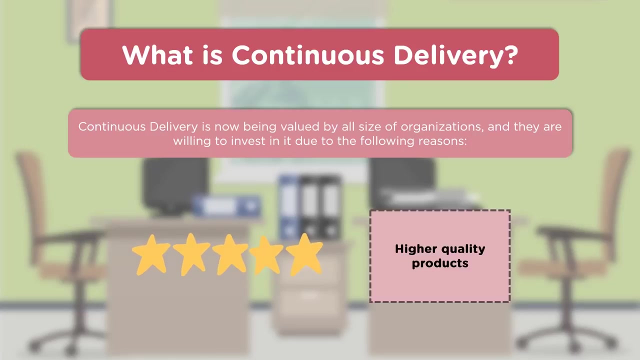 we will be able to deploy to pretty much any environment which we feel as such over here. So that's the real beauty about the continuous delivery: where we can actually deliver it to whatever environment we feel we want to deliver. Now, continuous delivery is also something which is a very important concept for most. 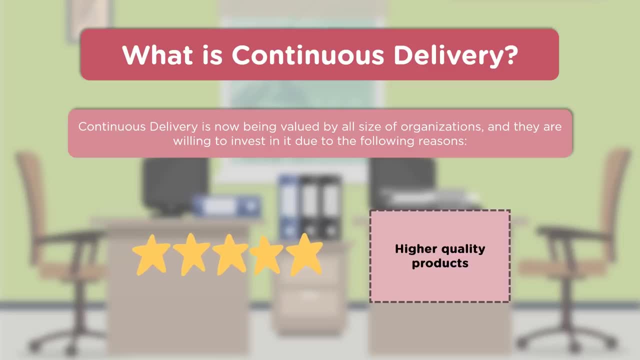 of the organizations. So each and every organizations are actually looking forward to invest in this one for a variety of reasons, because it's something where we can invest some of our particular efforts. budget money, a lot of things are there, But the kind of benefits 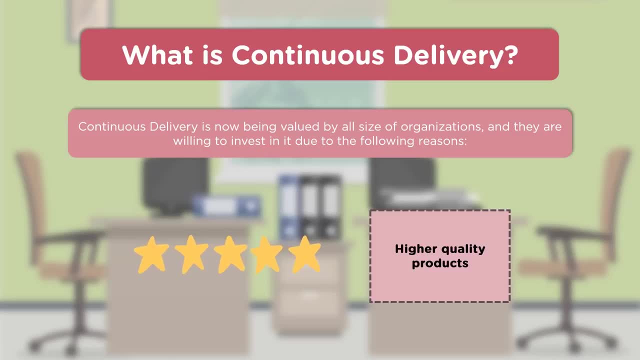 Which we get in the return. That's what we are going to talk about over here as such. So let's go with that. So it provides the higher quality of products. Yes, the efforts are there, Yes, that investment is also there, But in the return, the prime, the very important concept or very important thing which we get. 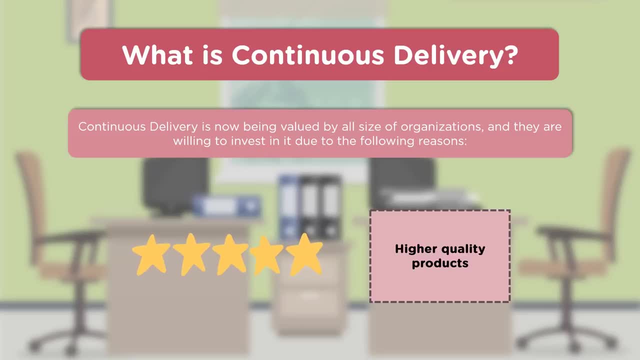 is the high quality of products here. So the kind of quality which we are getting with this one is quite high and that's the biggest benefit which we get when we talk about any kind of continuous integration, continuous delivery, So our continuous deployment here. So the quality is always top notch when we work of these particular processes. 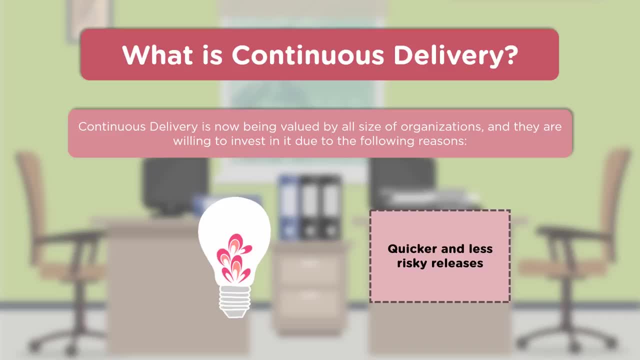 It also helps us to go for a quicker and less risky releases, So that's another benefit which we get this process. Customers are also satisfied because they feel that, yes, we are going with this particular automated process. within a few days, we are getting the deliveries. 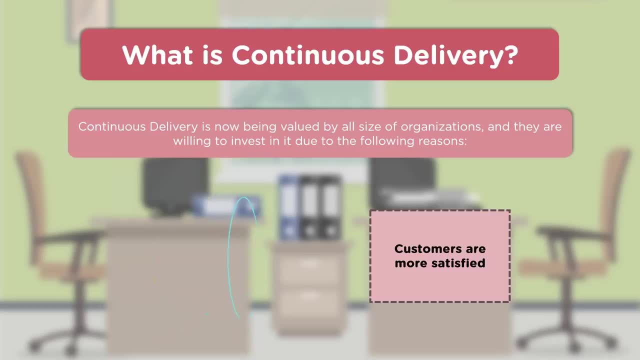 We don't have to wait for months for getting our delivery. so that's the biggest benefit which a customer usually gets when he talks about the continuous delivery, and it's more efficiency is there, and the cost effectiveness of the team also. So from the cost and from the particular efficiency, all those parameters are fully fulfilled when 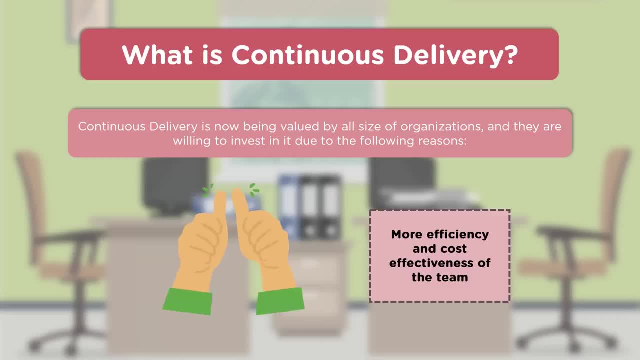 we talk about the continuous delivery. So this process delivers a lot of benefits which can eventually help us to go for a perfect, high quality product which we can develop as such over here. Now the next thing is the continuous delivery, Continuous deployment, which is an automatic deployment to the production environment. 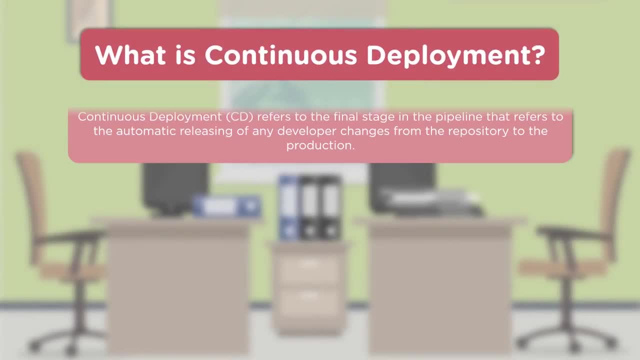 So let's see that. what exactly is in continuous deployment all about here? So continuous deployment refers to the final stage in the pipeline, So which means that we are not only preparing our artifacts, we are not only doing the particular compilations or test case executions, we are actually going one step ahead, and this one. 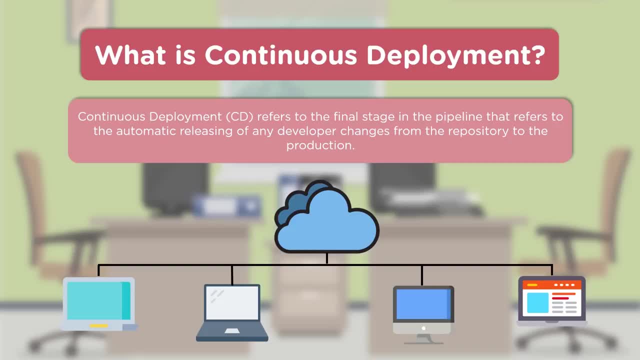 step ahead is nothing but the deployment to the production environment. So this is what we are typically doing when we talk about the continuous deployment over here: that we are going to one step ahead and that's where we are going for the deployment of our particular artifacts. 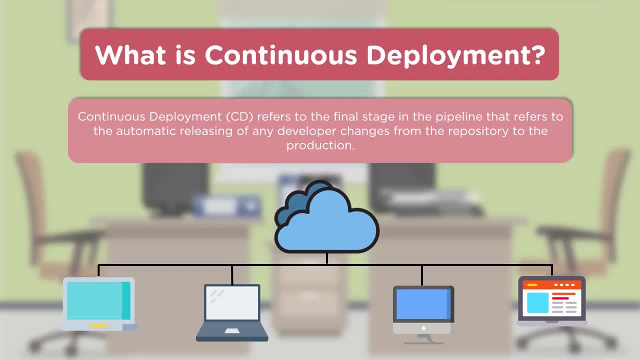 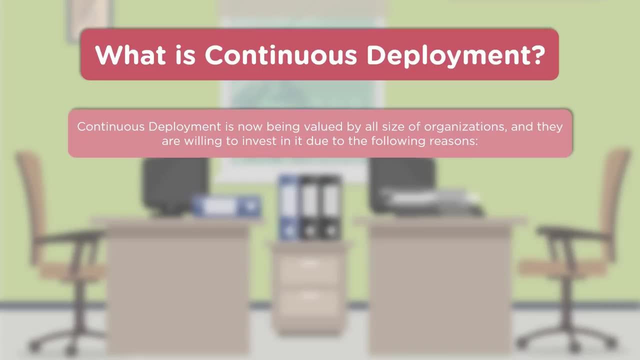 So we are deploying to the production environment so that our changes, whatever the changes we are trying to do, we are trying to make that should be deployed to the production environment Right now. so continuous deployment again is can be deployed to hire. whatever the organizations want to feel or want to deploy, they can actually go with that and there are a lot of benefits. 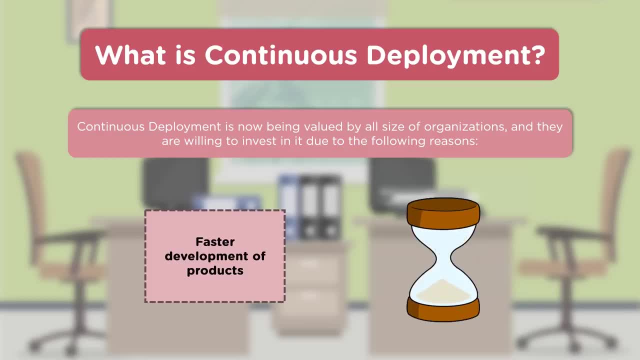 actually, which we get when we talk about the continuous deployment. So let's see about all these particular deployments one by one. So, first of all, the faster development of the products is there. So we are looking forward that when we are going for the automations, when we are going 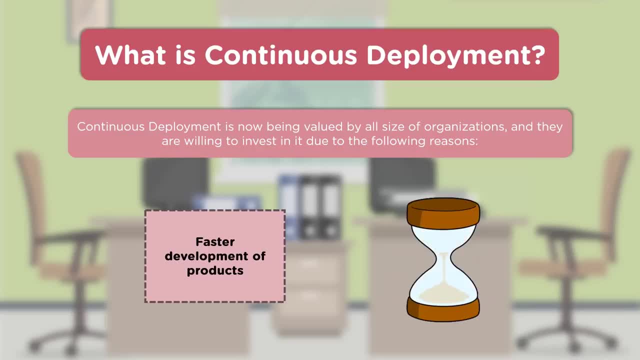 for this deployment. so if we get a kind of a faster- you know- development process which is there, so the products are getting developed very quickly, very fast, that's the biggest benefit which you are getting when we talk about this continuous deployment here, And it's less risky releases also there and it's easy to fix problems, whatever the automations. 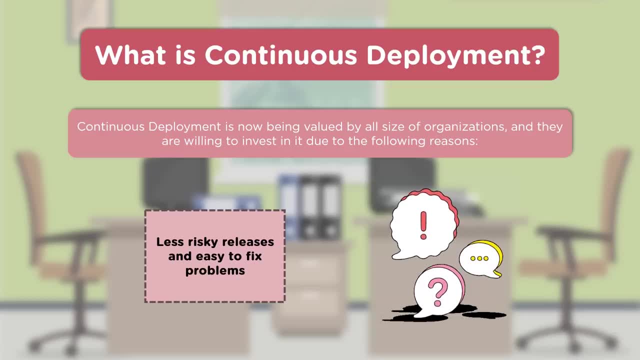 we are feeling We are trying to perform, that can definitely help us to go, that how we can automate and how we can go for this particular releases over here. So these releases are very less risky because we are doing all the things automated. There is not much of a scope, which is there for the manual errors. 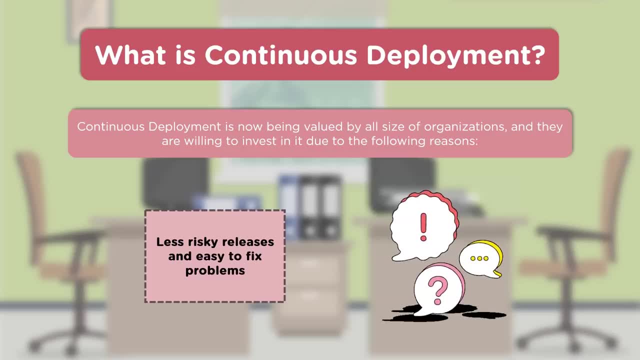 So usually manual errors is something which is the biggest problem or which is the biggest risk when we go for any release, But that is something which is totally removed with this automation here Now. it also helps in continuous improvement in the quality, So continuously improve quality is also getting improved as such here. 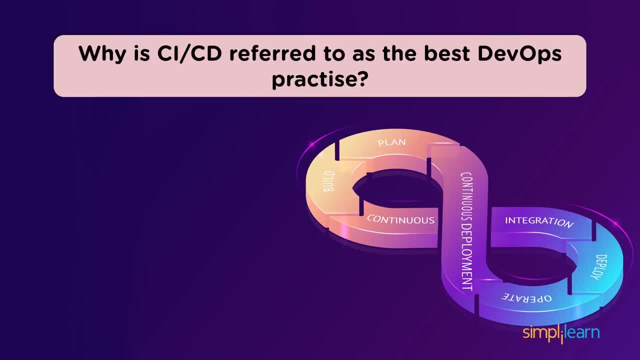 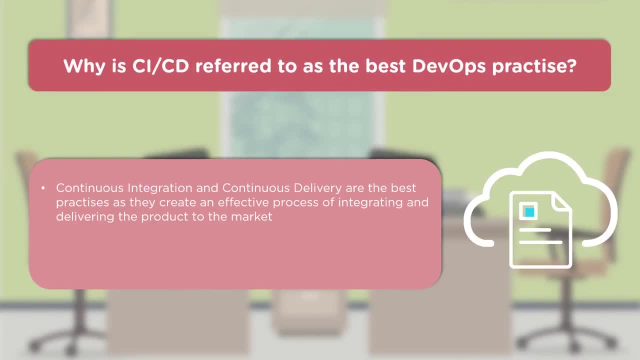 Now, let's talk about that. why, exactly as- and we talk about at the industry level, in the market level also- that the CI CD is one of the best practices. Now, what is the reason behind that? Why those are known as the best development and devops practices as such. 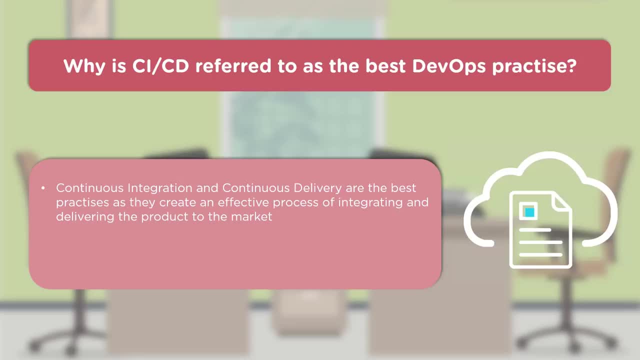 Now, continuous integration and continuous delivery are the best practices, as they create an effective process. the kind of integration and delivering the source code. These are the prime things which we need to take care when we talk about the development teams over here. So they want an automated process first of all, and they also want to streamline process. 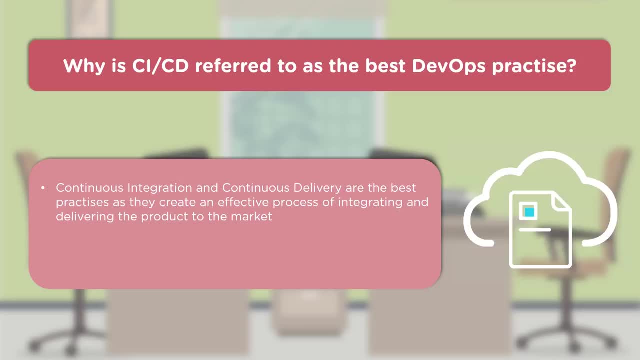 which can you know, take up the things which should not fail. It should be a failsafe process mechanism through which they can release various kind of changes to the production environment because ultimately, they are looking forward for the deployment of the changes to the production environment. 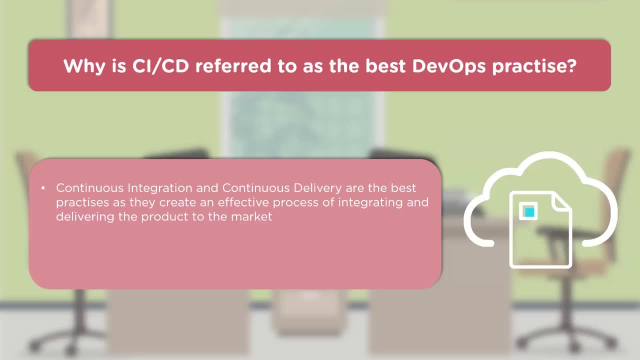 So how they are going to do that. That is where the CI, CD, Or the continuous integration and continuous delivery, helps on that part, And that's the reason why they can help the teams, the development teams, to go for an effective process implementations when we go for these implementations of these two practices. 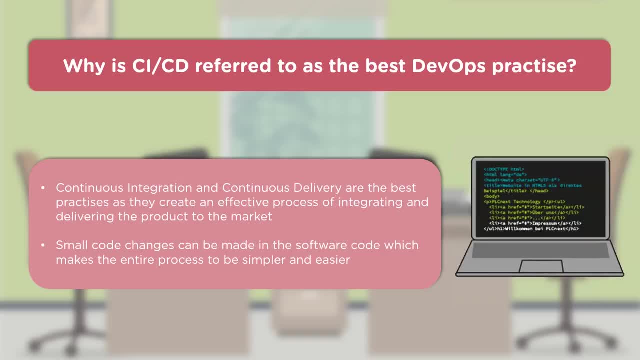 Small code changes can be easily made in the software code, so you don't require much of the efforts if you are going for even small changes in the source code that can also be effectively deployed to a production environment in a simple, straightforward and easy mechanism. the changes can go from the developer machines to the production environment. 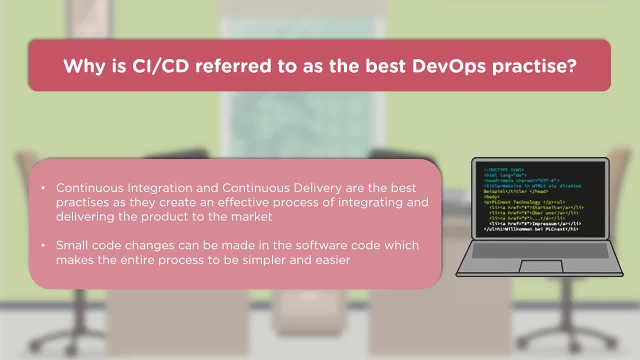 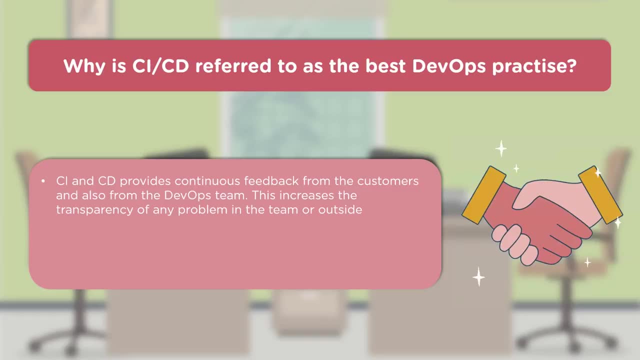 That's the biggest benefit which we get, due to which we feel that, yes, these two processes should be implemented into a devops platform, right. So CI and CD provides continuous feedback from the customers and also from the development teams- devops teams, So the increase of transparency is also something which is important, which is implemented with. 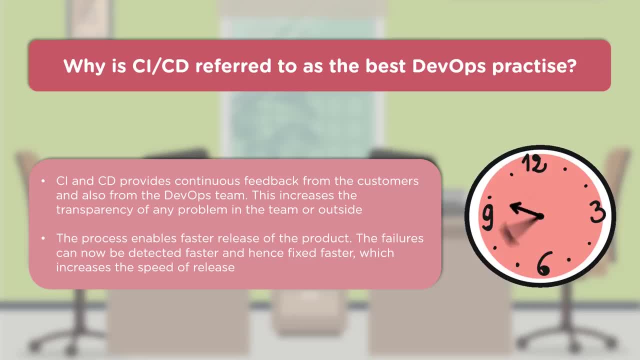 these processes here. So the process, It's faster release of the product. So we don't have to wait for months to release the source code there. within a couple of hours, within a couple of days, we can actually release it to the production environment provided.